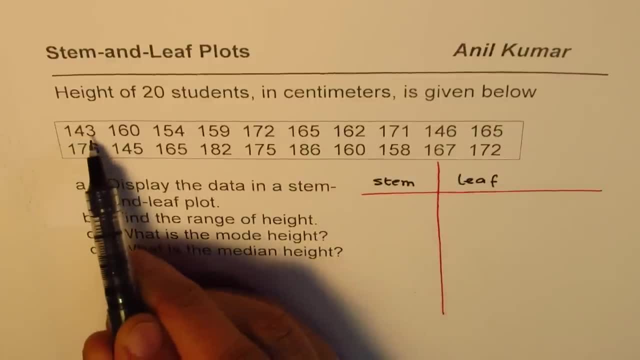 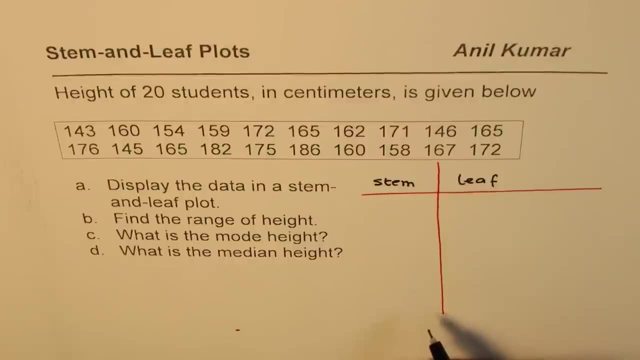 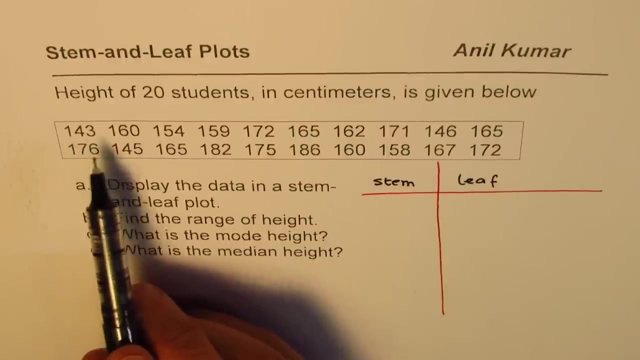 In leave we'll be only writing the one's place right. So number here, for example in one's place, will be written in the leaf part right now, before entering the values, we should kind of have a general view of the data. it starts from 1, 4, 3, and highest number seems to be 1, 8, 6. so 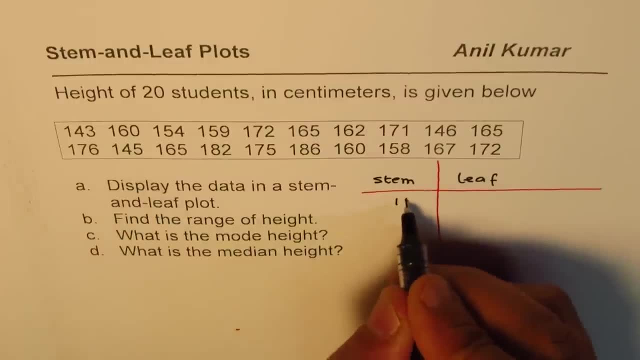 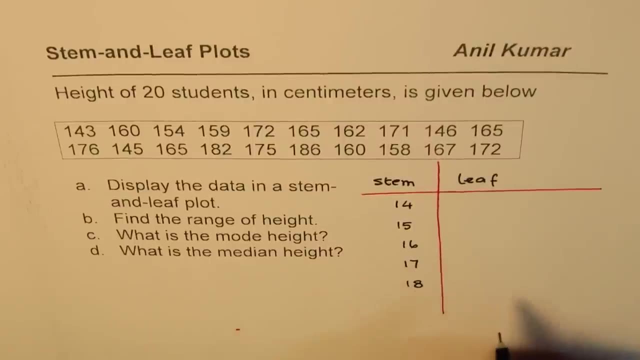 that means in stem we have numbers like 14, 15, 16, 17 and 18 curry. so looking at highest number and the lowest number provides us the range in which these numbers are going to be arranged. so now we'll just take numbers one by one: 143. 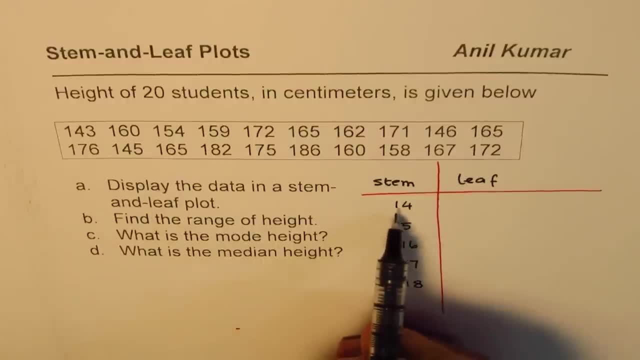 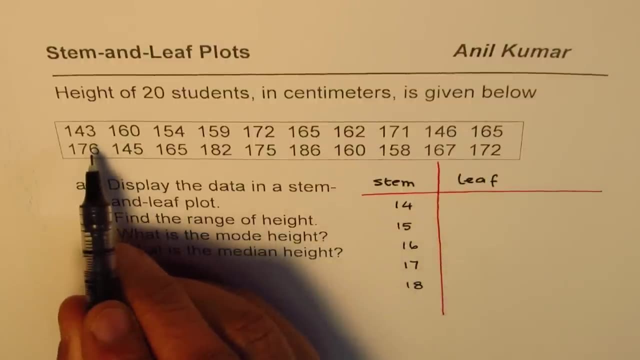 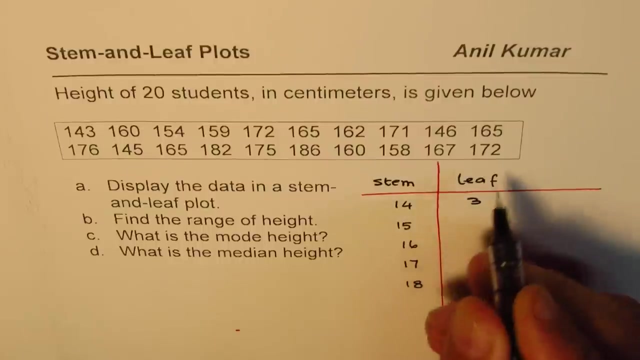 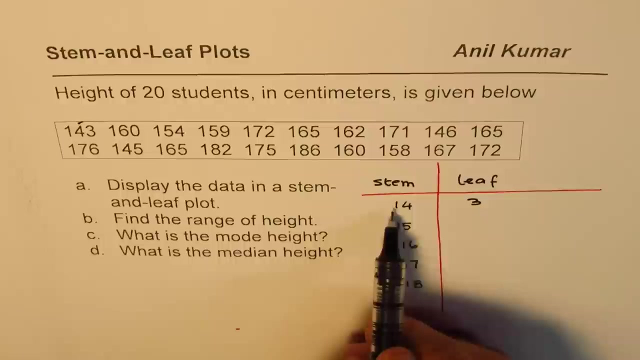 now 14 is 110 and 3 is once place. so 3 will be written in the leaf part. now when you write 3, then we should try to arrange them in increasing order. so I'll write 3, kind of leave some space for 0, 1, 2, if any right. so what? we'll move on a sequence in a sequence, always 143. so this is 1. 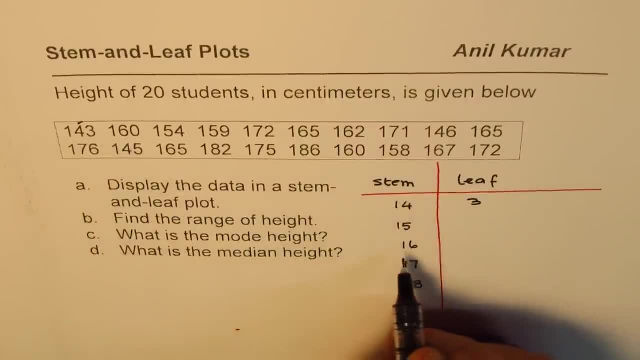 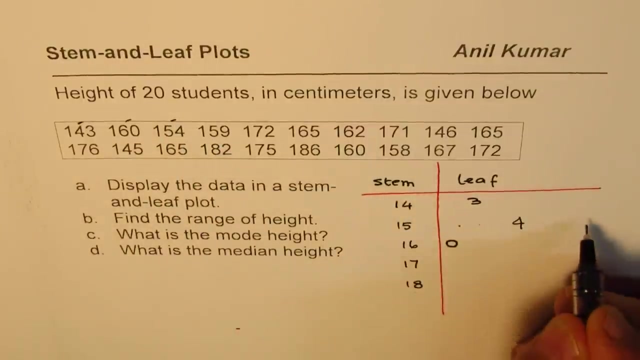 4, 3, 143, 160 means 1, 6, 0, right 154, 1, 5. I'm writing 4 slightly away because there could be other numbers on the left side of 4, right 159, so I could write 9 almost at the end of my column. okay, so this row of 15. 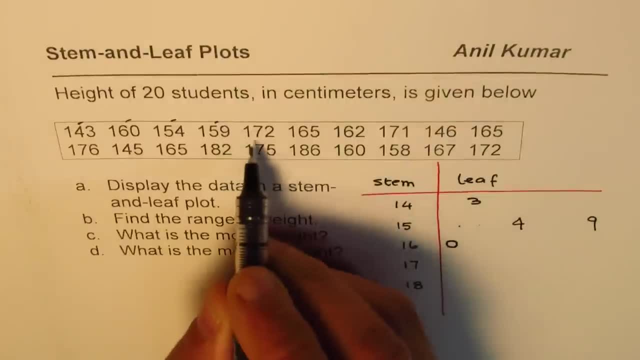 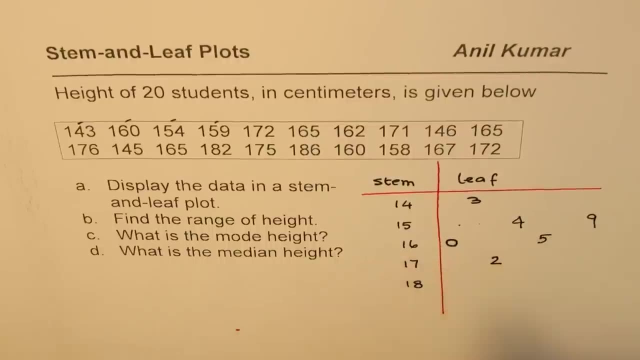 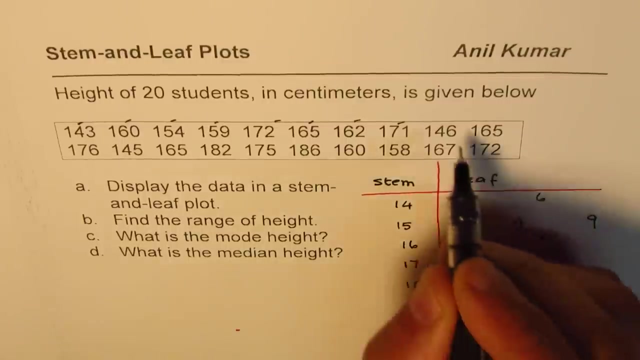 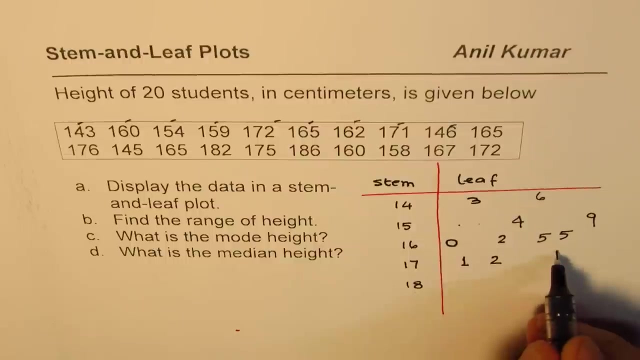 I'm writing 9 almost at the end: 172, 1, 7, 2, okay. 165 1, 6, 5, 162, 1, 6, 2, 171 1, 7, 1, 165, 1, 6, 5, 176 1, 7 less is 6. 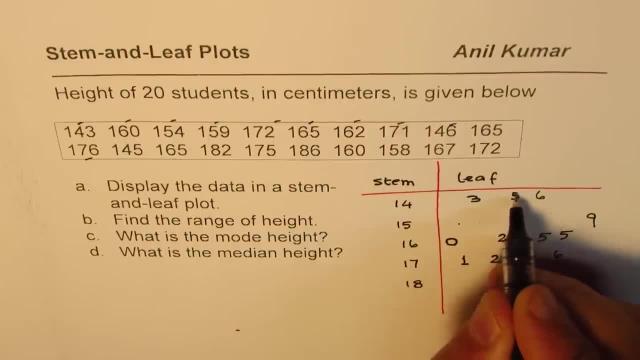 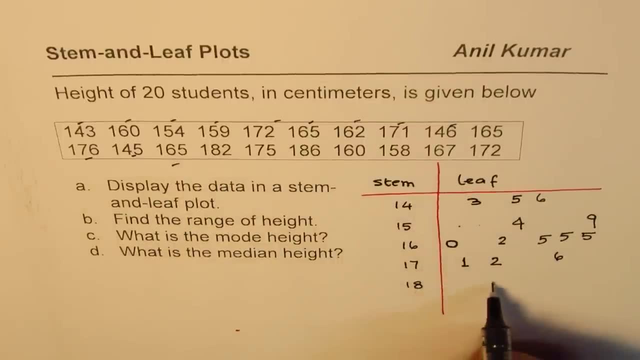 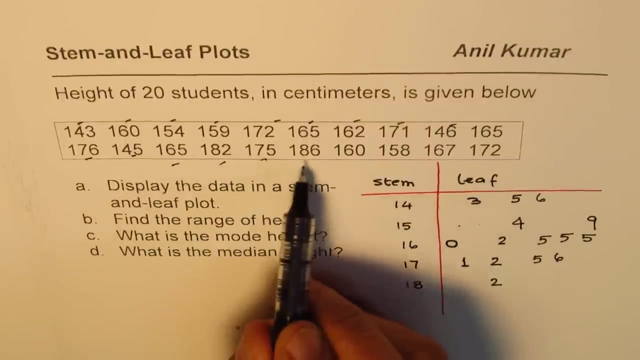 145 one 4, 5, 165, one six, 5, 182, 182, 175, 175. you see how am I in arranging these numbers in increasing order. it is kind of necessary, right? so 175 is the last number one. eight six one eight six one. six zero one six zero. 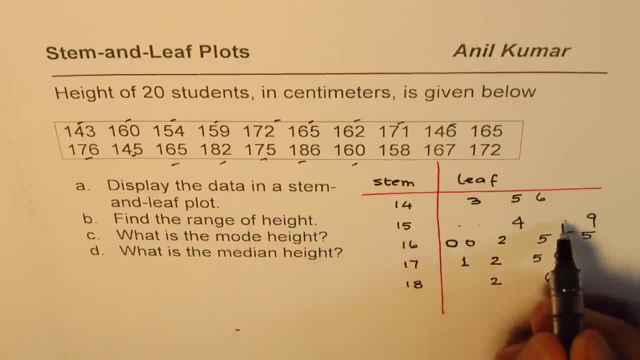 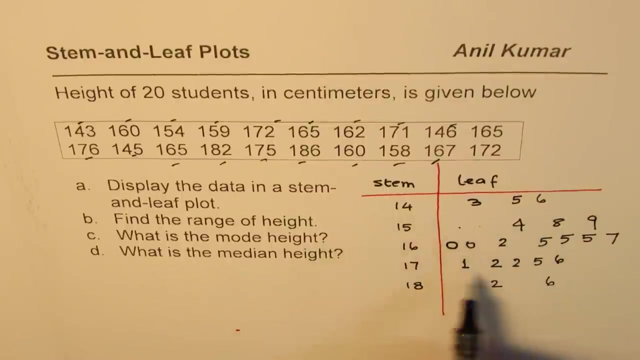 one five eight, one five eight, one six seven, one six seven and one seven two, one seven, two, right. so we've kind of filled up and that is how our leaf, stem and leaf could plot looks like. well, sometimes you may be required to make another copy of it so that you could write these numbers nicely. 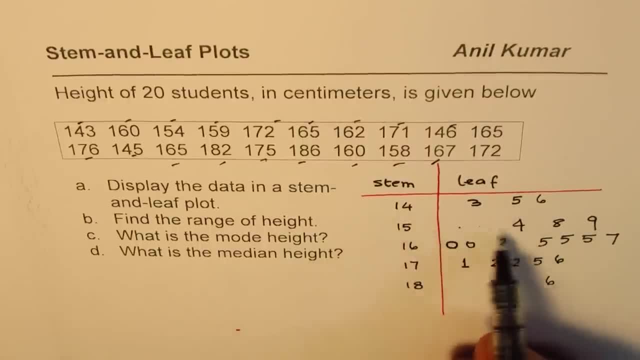 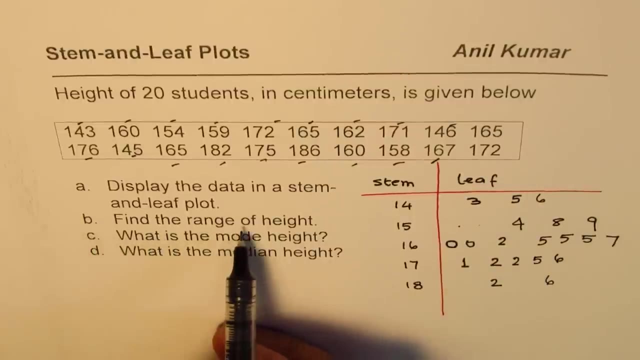 right. so one-fourth, three, five, six, a bit closer than four, eight, nine anyway, but this will also work for you. now let's look into part B. so leaf stem and leaf plot has been drawn. part B is: find the range of height range. what do you understand by range? range is the spread of data. it is maximum take away. 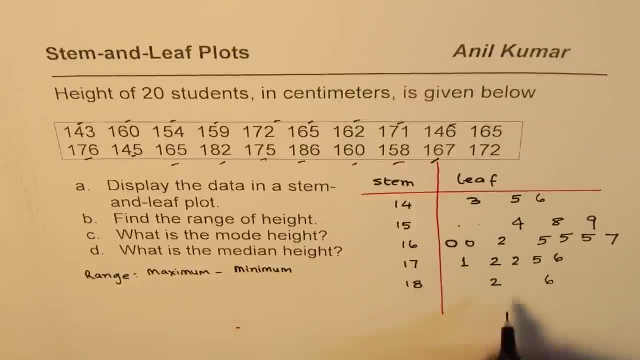 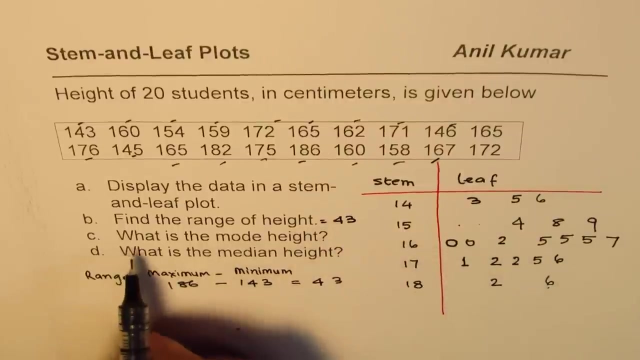 minimum. so in our case maximum is 186. do you see that 186? take away minimum, 143, 143, and that gives you six. take away three is three, eight. take away four is four, so we get 43 as the range. so the range is equal to 43.. what is the mode height? mode height means most frequent, so we can. 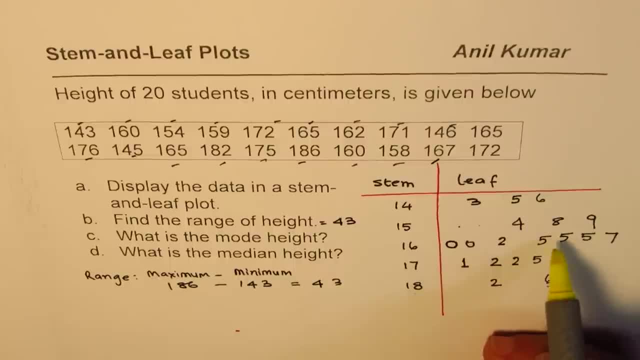 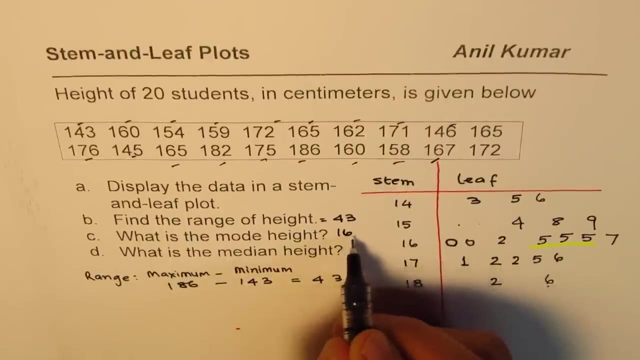 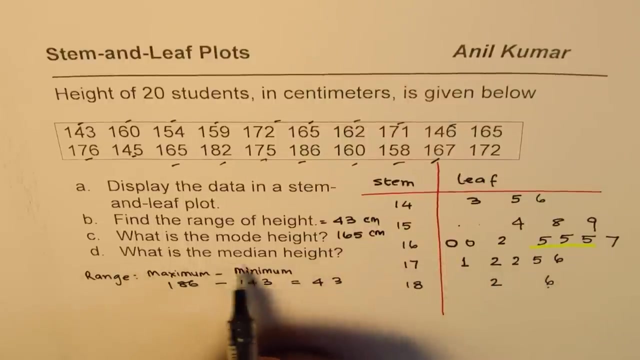 so we can look into leaf part and see which number repeats most in any particular row. so here, five, we got three fives repeating for one six. that means 165 is most frequent height. so it is 165, right. and of course all this is in centimeters, right, so you can write centimeters. what is the median now? median? 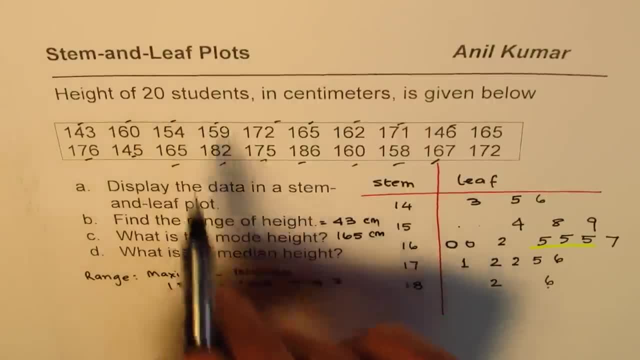 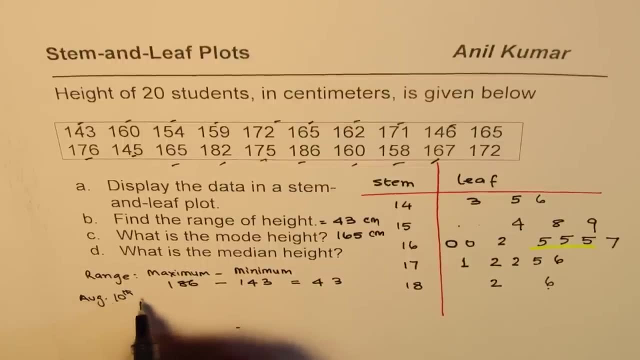 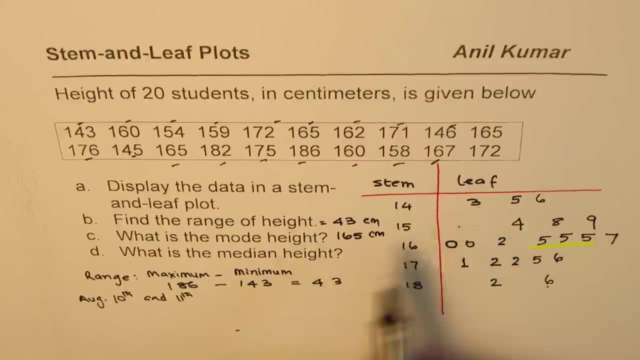 is the center value, since we have students average of 10th and 11th. so average of average of 10th and 11th right will be the median, so let's count. so, once you arrange them in increasing order, as we have done, count the 10th and 11th position: 1, 2, 3, 4, 5, 6, 7, 8, 9 and 10. 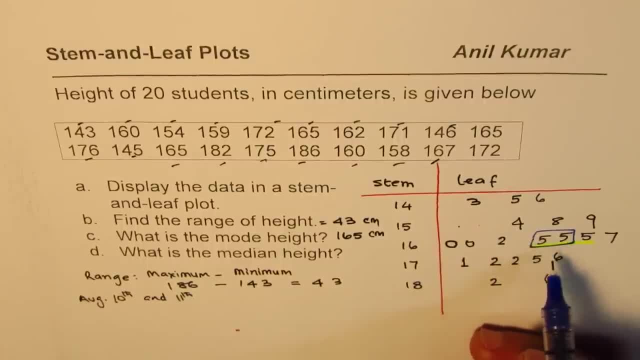 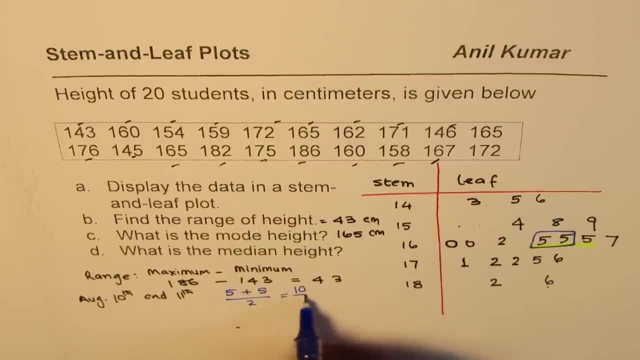 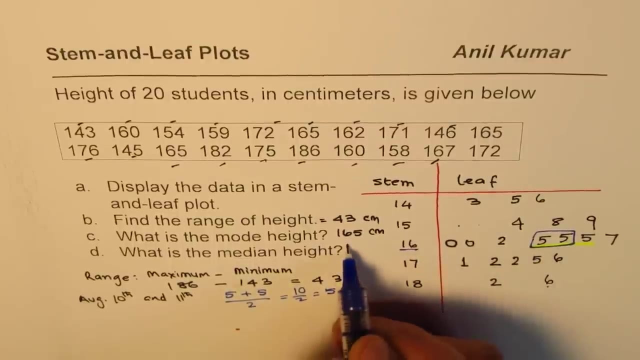 and 11, right? so these are the numbers: 5 & 5. average of 5 & 5 will be 5 plus 5 divided by 2, which is 10 divided by 2 or 5, right so? so the median will be 1, 6, 5. so 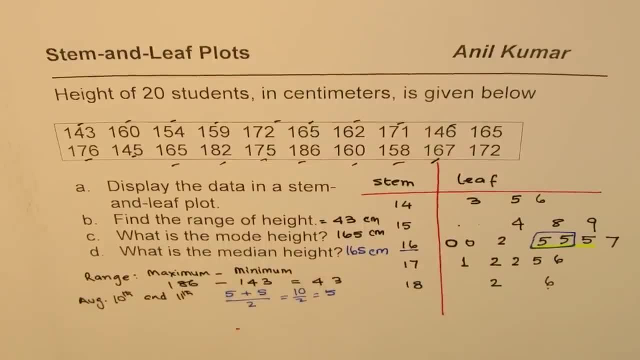 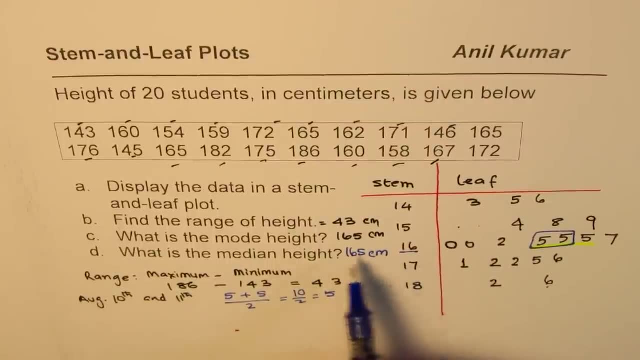 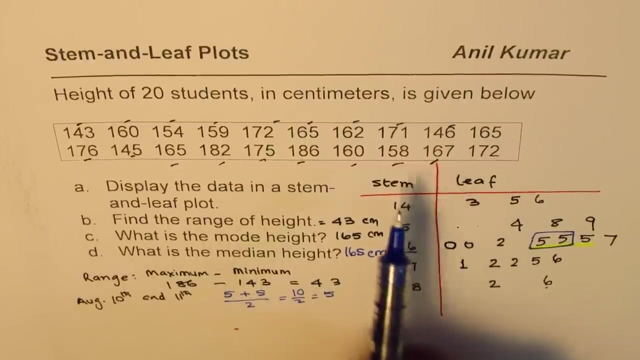 we have 165 centimeter as the median in this particular case right. so that is how very easily we can find all these parameters for measuring, spread or averages, with the help of stem and leaf plot. now here is a question: if you draw a histogram with this data, will you be? 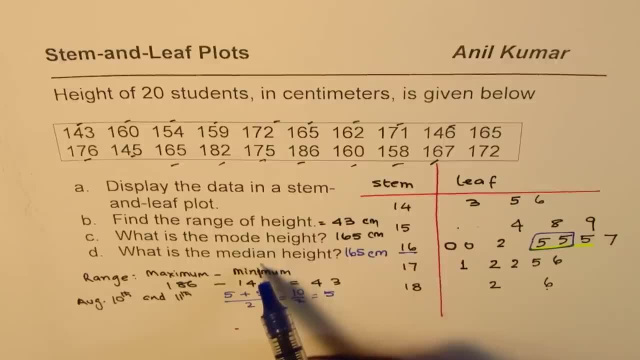 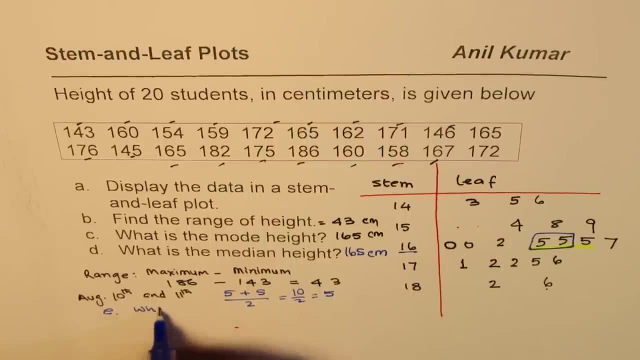 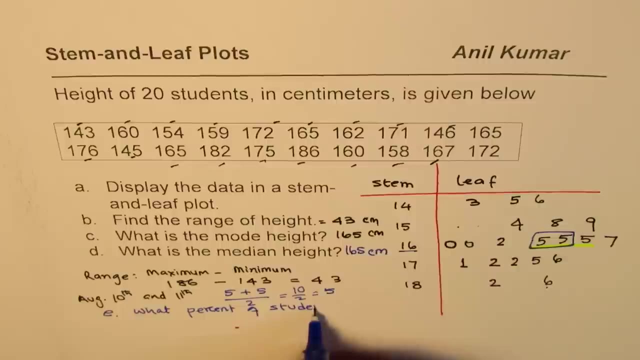 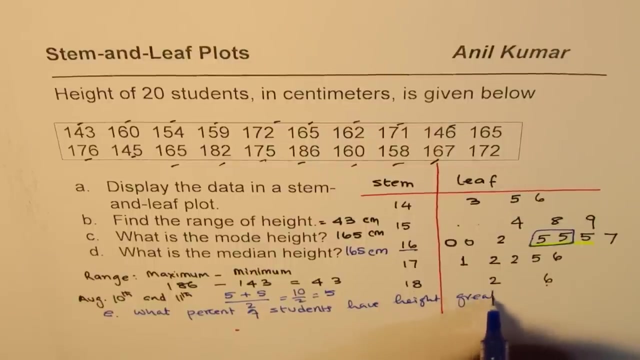 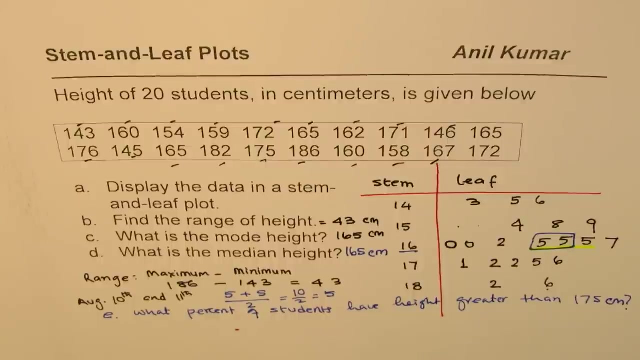 in a position to answer these questions. think about it and answer. now. here is another question for you: what percent of students, what percent of students have height greater than 175 centimeters? so that's the question for you. can you answer percent? remember, we have to divide by total number of. 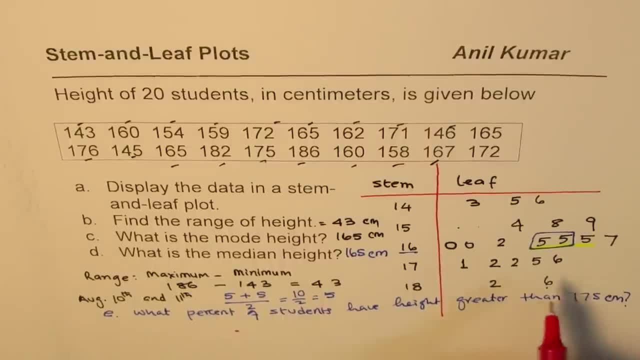 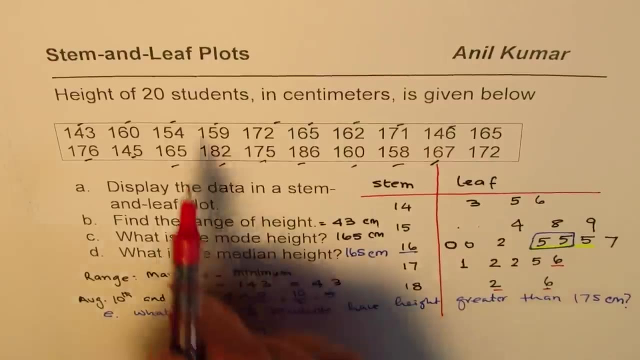 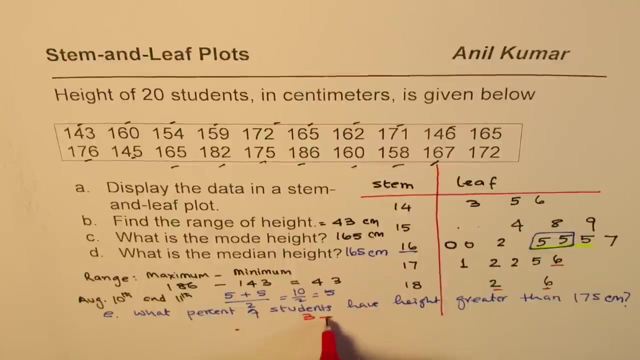 students. okay, so let's answer this. greater than 175 means these three students, 176, 182 and 186. these, through three students, have height greater than 175. to find person, it will be 3 divided by total number of students times 100, correct? so it'll be 3 divided by 20 times 100, which is 15. 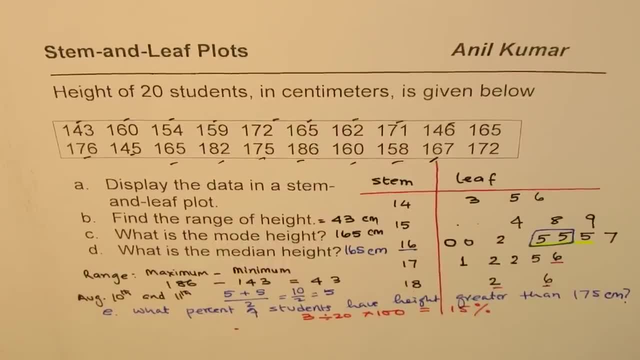 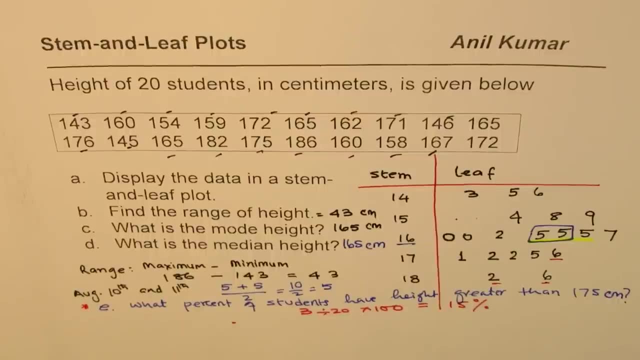 right. so 15 percent students have height greater than 175 centimeters. so this is a very important question to understand and we can answer all these questions from stem and leaf plot. if you draw a pie chart or a histogram or a bar graph, you'll not be in a position to answer these questions. 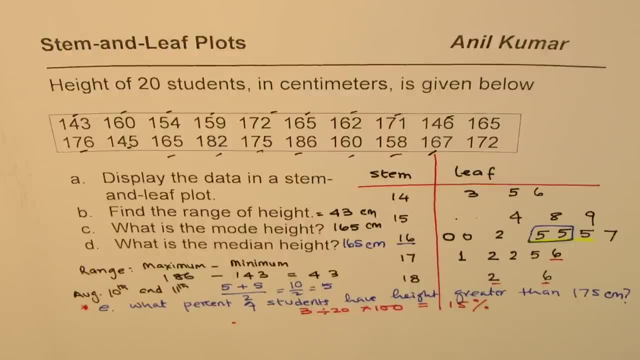 which we have discussed, and that is a huge advantage of stem and leaf plots, Amanil Kumar, and I hope you have greater appreciation for this kind of representation of data. you can always share and subscribe my videos. thank you and all the best. 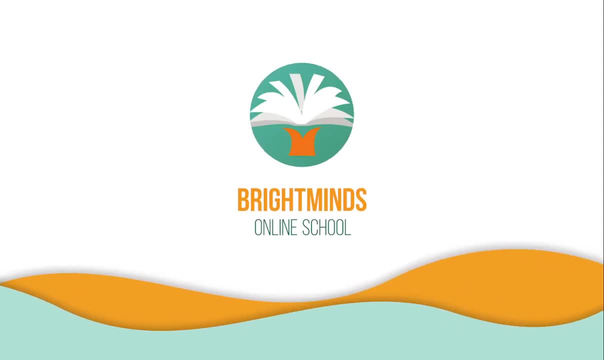 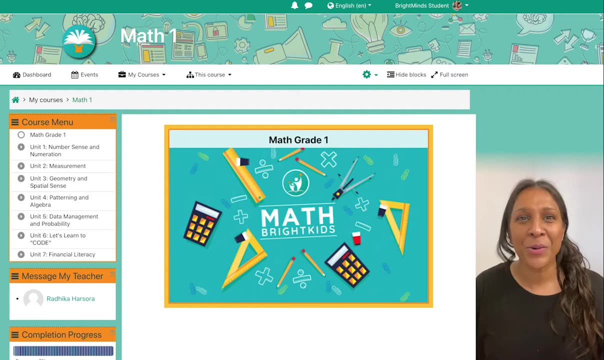 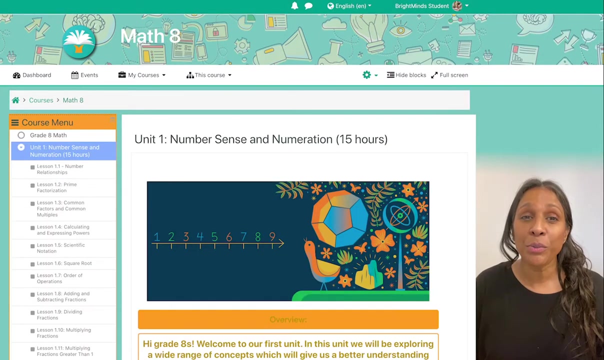 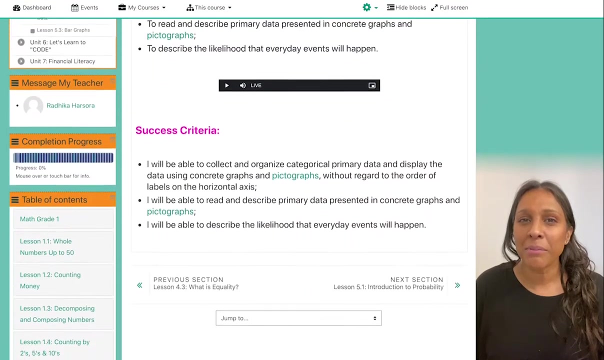 Welcome to Brightline's online school. Here's an introduction to our elementary math courses. Throughout our math courses, students deepen their learning through seven areas: Number sense and numeration, measurement, geometry and spatial sense, patterning and algebra, data management and probability. coding and financial literacy. 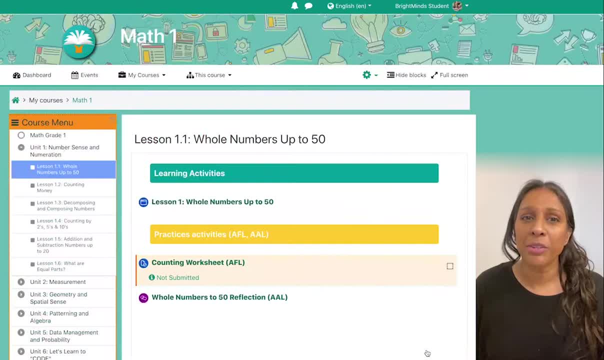 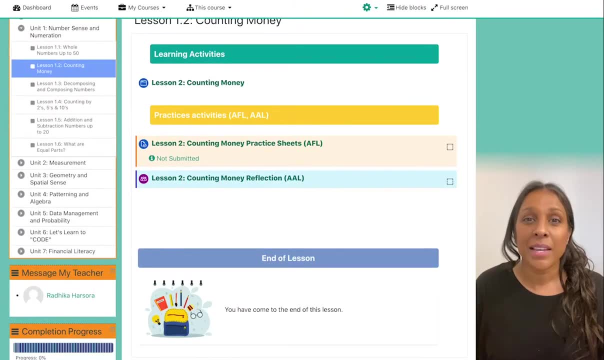 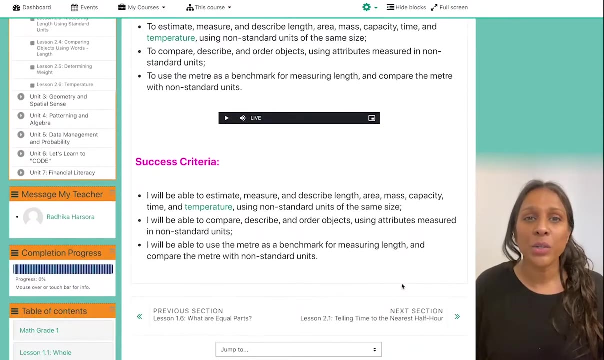 Throughout our math courses, our students will develop their understanding of numbers and their operations in order to solve problems with different strategies. This math course gives students the tools to work with non-standard units of measurement in earlier grades, eventually working with the basic metric units to measure different quantities later on during their learning. 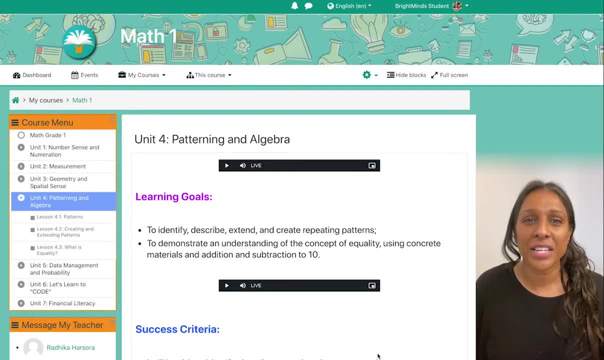 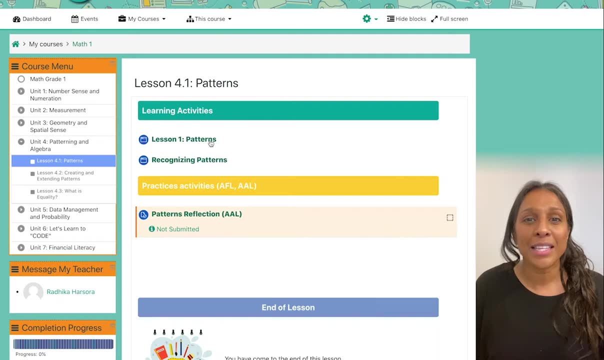 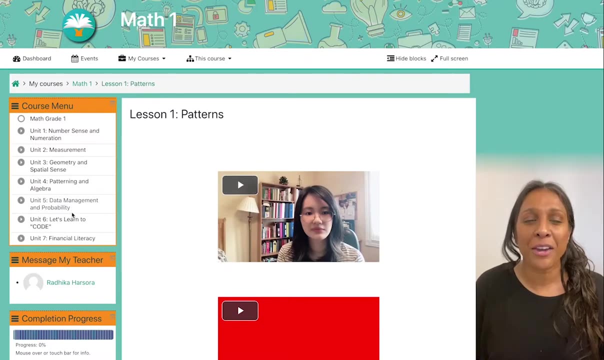 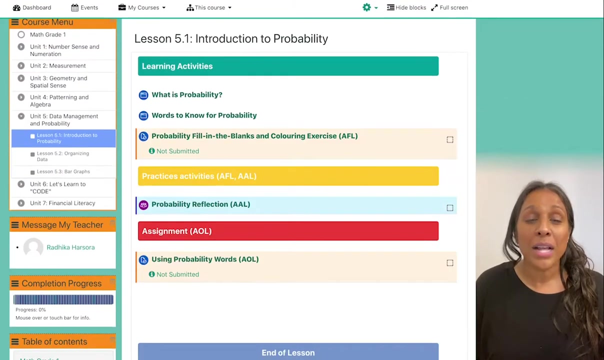 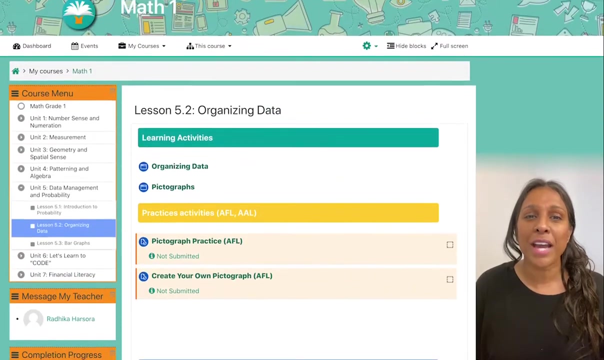 Students will learn to identify basic shapes and figures in order to recognize and compare their geometric shapes. We will work with patterns in this course and ways to extend them, working towards graphs, tables and verbal descriptions to generate patterns in older grades. Students will also learn how to gather, organize and display data in younger grades, while developing their analyzing techniques to further their understanding of the data being presented to them once they graduate to older grades.